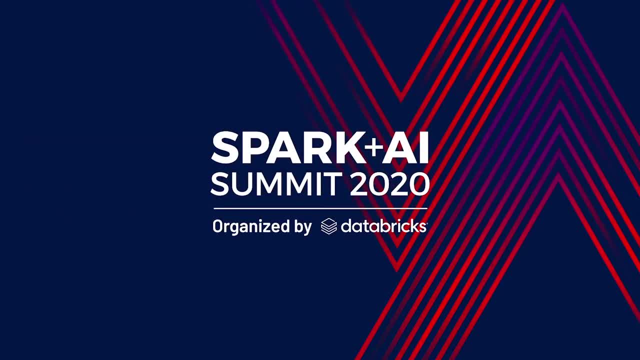 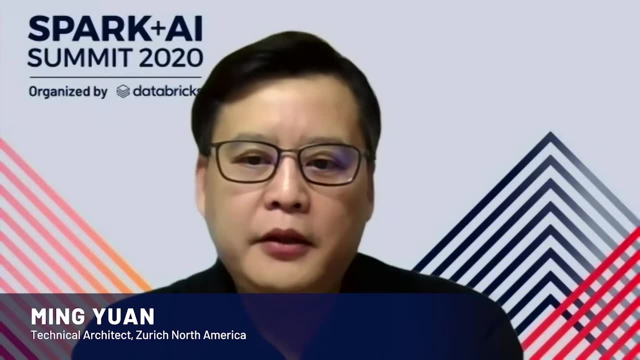 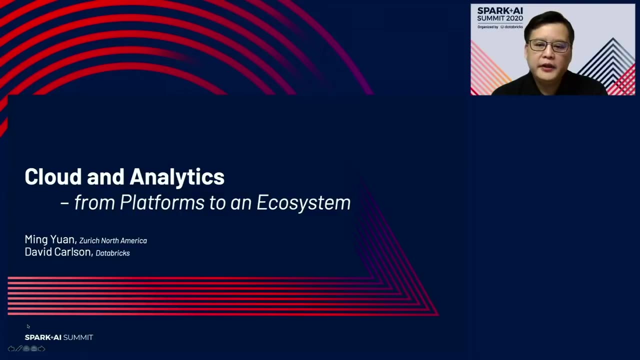 Hi, good afternoon. Thank you for attending our session. My name is Ming Yuan, I'm a technical architect working for Zurich North America, And today, Dave and I, we are going to share our journey of building an analytical ecosystem on the cloud. So now turn it over to Dave. 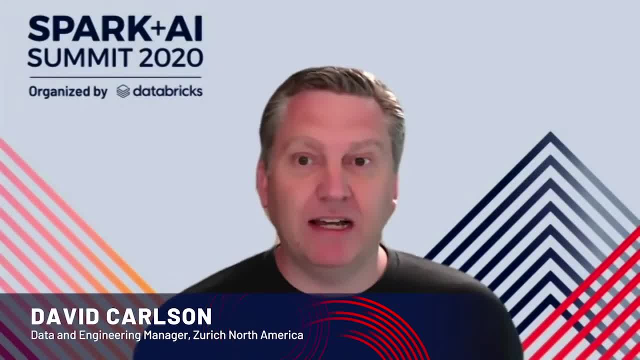 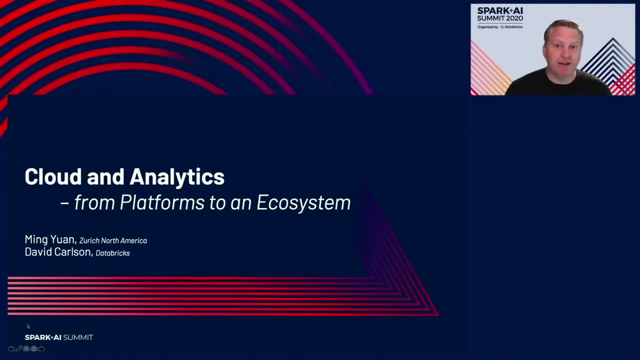 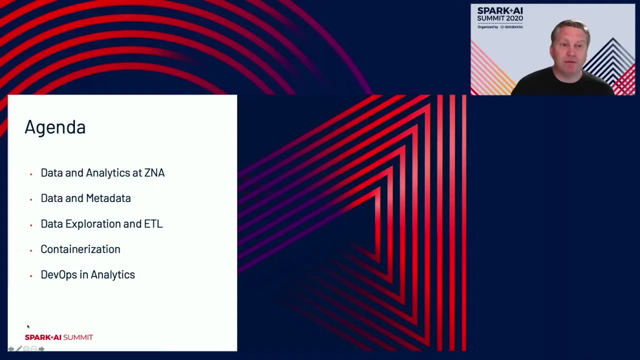 Hi everyone. I'm Dave Carlson. Currently I'm a solutions architect at Databricks. Formally, and that's what we're here talking about today, I manage the analytics and engineering team at Zurich North America, So today we will be talking about some of the technical capabilities. 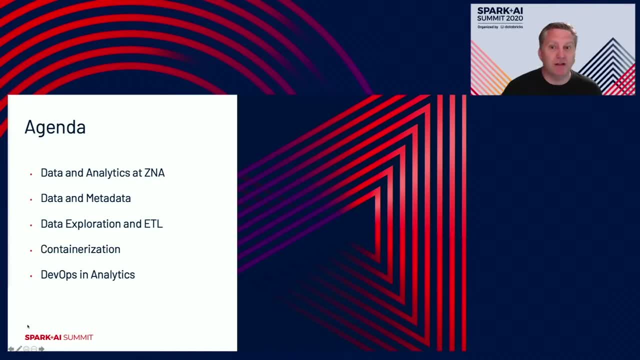 that have been built out at Zurich and how they support the end-to-end analytic lifecycle, And Ming will kind of go into some detail around our meta store as well as some deployment capabilities that have been built out. So for those that are not familiar with Zurich, North America. 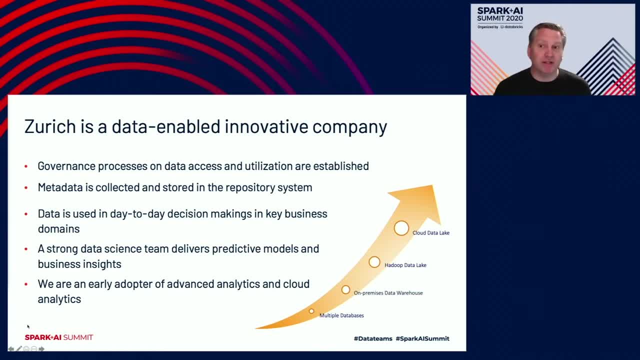 we're one of the largest commercial property and casualty insurance companies in the US And we're part of the larger global insurance group. So the area that I worked in was called data analytics, And one of the things that we wanted to do was build an analytical ecosystem. So the first thing we did was build an analytical ecosystem. So we got over 50% of our data and we built over 50% of our data. So we got over 50% of our data and we built over 50% of our data. 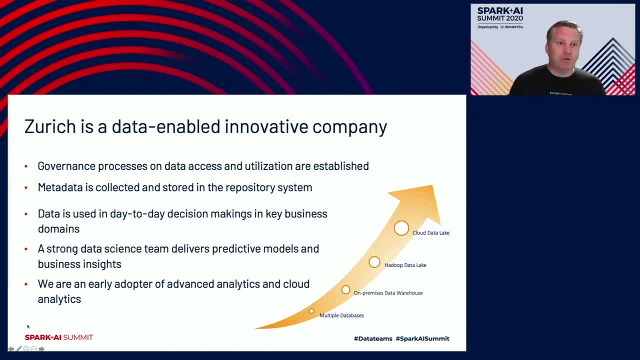 And we built over 50% of our data. So we built over 50% of our data And we built over 50%. We built over 50% of our data. wanted to make sure we could do, is you know, really make sure we could, you know? 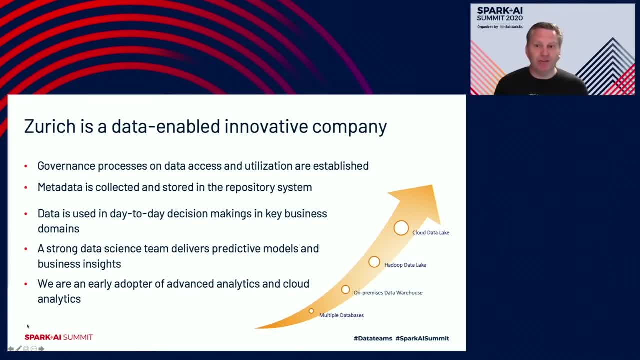 bring you know data-driven decision-making. you know to our business and you know at Zurich there are three main focus areas that we have. you know customers, you know we want to make sure you know through like that, our data insights so you know we can help our customers. you know, better understand and 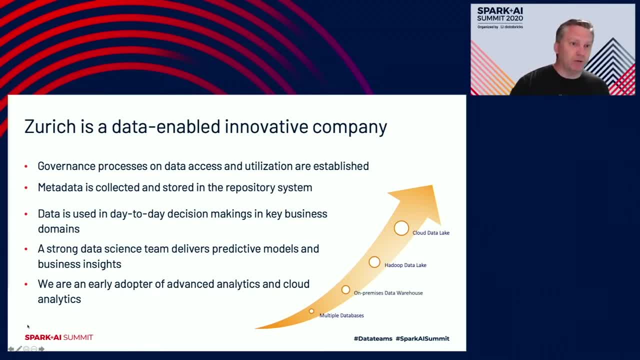 manage their risk, you know. so you know the best. you know. you know loss is one that doesn't happen, right, you know underwriting. we wanted to make sure we could support and enhance the risk selection process, you know, be able to help our underwriters and our business leads, you know, with their program. 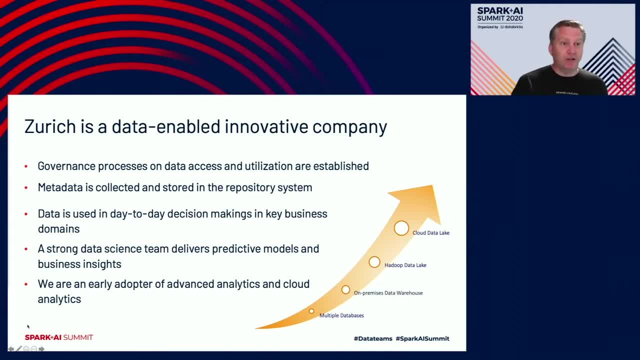 structuring and you know pricing decisions, both at an account level and also at a portfolio level. and, last but not least, claims. you know we want to make sure we could improve. you know outcomes. you know in the claim handling process. you know, so make sure you know claims that potentially could. 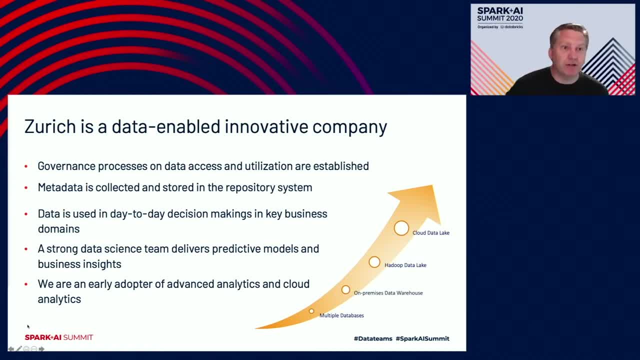 develop, you know, into more severe claims without proper over-examination. and then you know, you know we want to make sure we could oversight. you know we get the right place, professional maybe, and get, like a nurse practitioner, assigned on, you know, claims that may develop into more severe. 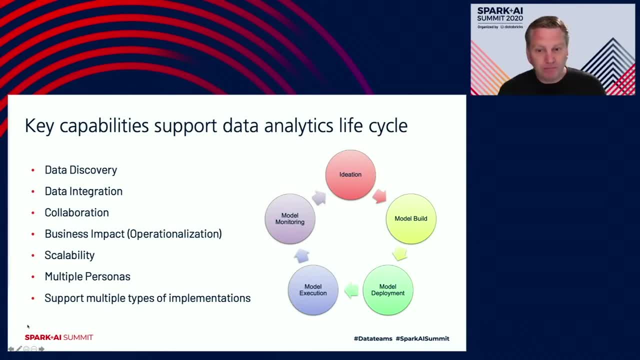 risks and you know how do we do that. so you know, to the right you'll see. you know many people have seen some iteration of you know the Alex life cycle from like ideation to your actual model, build, development, execution and find value in your time, all monitored, right. so what are some of the key? 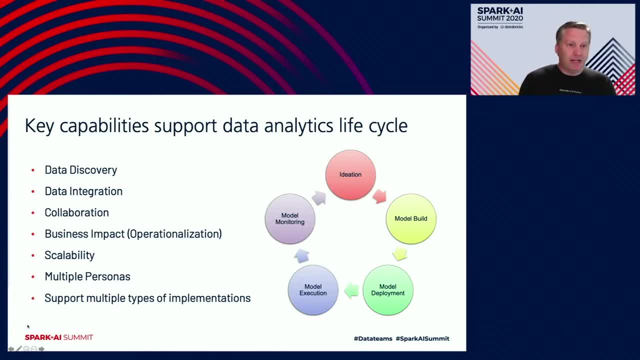 capabilities that we needed. you know because you know data scientists. you know what you need is. you know you need some fairly technical capabilities, but at the same time, you know you're not developers where, as data scientists, you know. so we want to make sure you know things that need to be taken care of. but 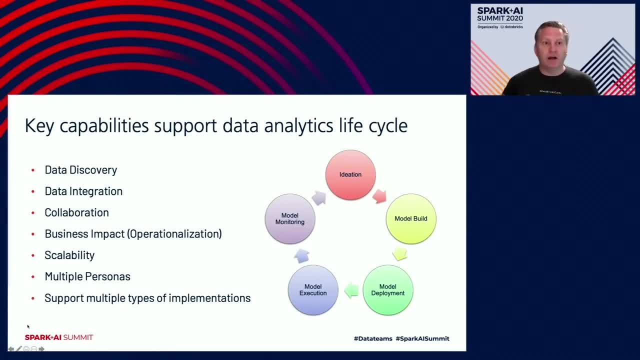 we don't want to be aware of day-to-day bases. like you know, securities scalability are, you know, taking care of for us? so you know some of the key. our data discovery: I know what I can analyze and what I can't analyze. I can't analyze what I can't find. 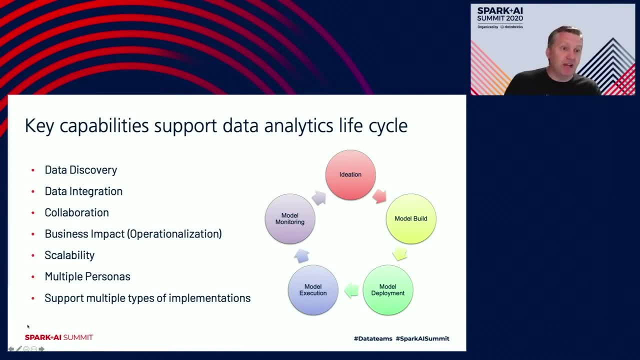 So we need to make sure, through the tens of thousands of tables we potentially had access to, that we could easily find and discover the relevant data needed for analysis and also be able to make sure that, once we discovered it, we're actually able to integrate it in a way. 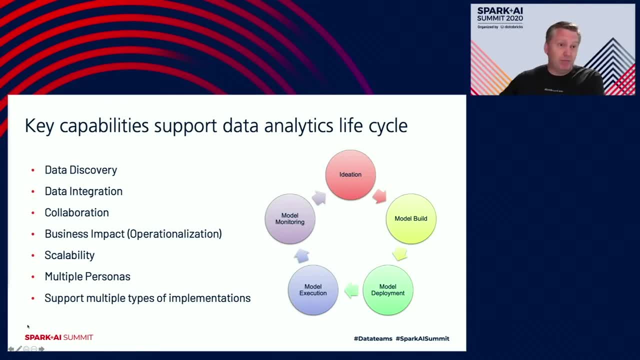 that we could actually potentially work with data engineers and build it out into something we could actually deploy in a data pipeline, Because previously we had proprietary analysis tools that we'd do the analysis and we'd have to extract all the business requirements and deploy it. 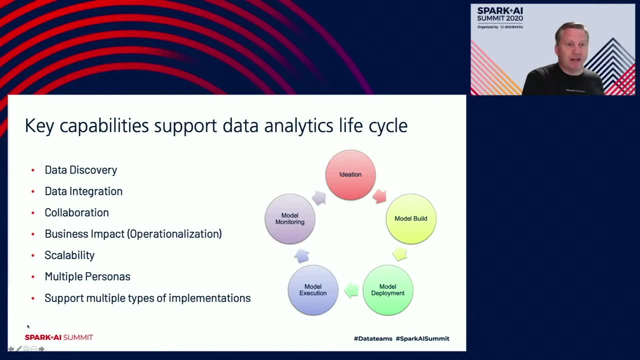 And that could take potentially up to two years. Back in the day, when we used proprietary tools, it had to be refactored into other deployable languages, So we had to have a lot of data scientists and data engineers in the same office and collaboration. 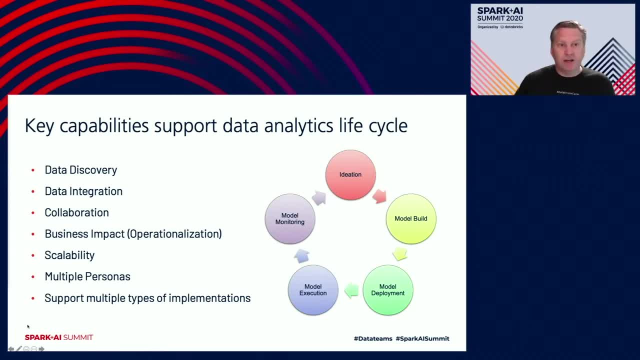 Not all of our data scientists and analysts are co-located in the same office, So we're not all in the same city country, time zone. So we need to make sure that we had a tool set that we could encourage collaboration on projects. 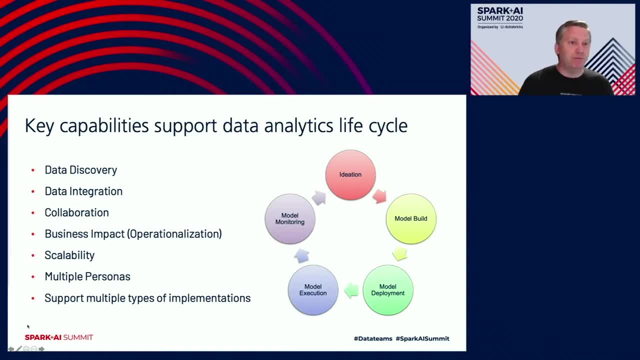 on multi-person teams, Not only multi-person teams, but also multi-persona teams, So we might have business analysts, actuaries, all wanting to contribute and understand the source of the data. what transformations are being done? are they being done appropriately? 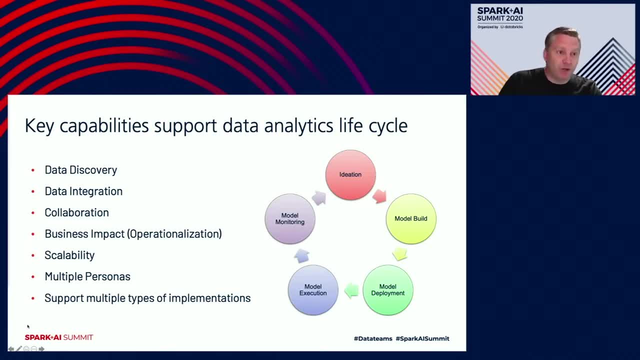 being able to try out new features and integrate them quickly. So that was one of our requirements as we were building out this ecosystem of tools and overall analytics landscape And, definitely not least, business impact. We want to make sure that we have a lot of data scientists in the same office. 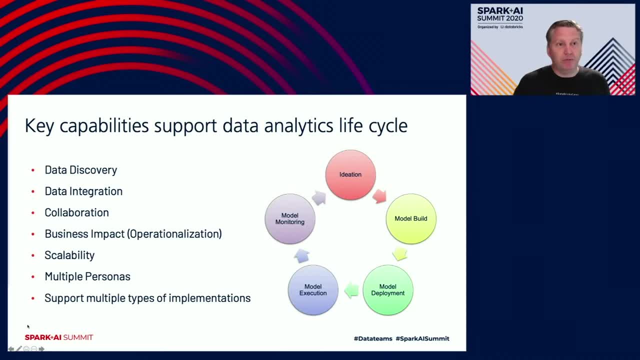 So we wanted to make sure that we could severely decrease the speed to market rate. So we wanted to make sure that our data discovery tools integrated with our integration standpoint to the extent if our data scientists want to use common data science frameworks in Python and R. 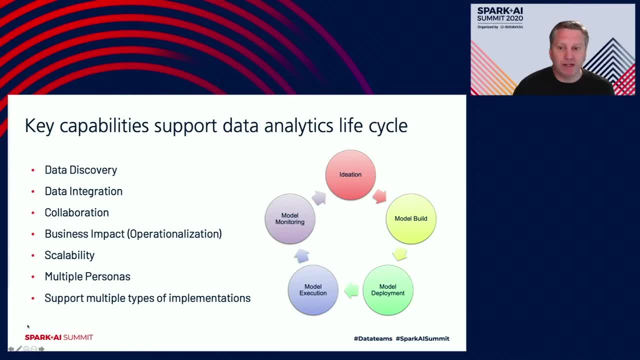 we could easily connect all of those together and chain them in a deployed pipelines, And so we wanted to make sure that we could severely decrease the speed to market rate. And so we wanted to make sure that we could severely decrease the speed to market rate. 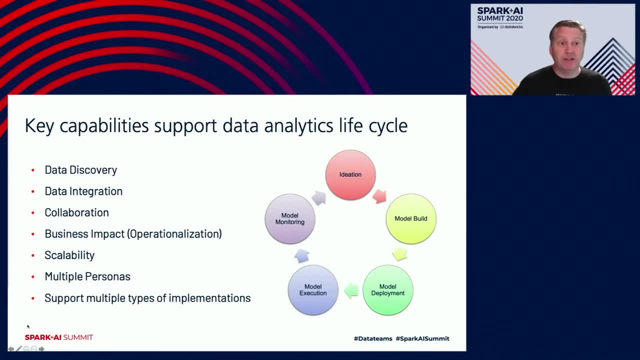 And so we wanted to make sure that we could severely decrease the speed to market rate. And related to that is multiple types of implementation. Sometimes we might be building something to integrate into a calling application, So we might have to build a REST API. 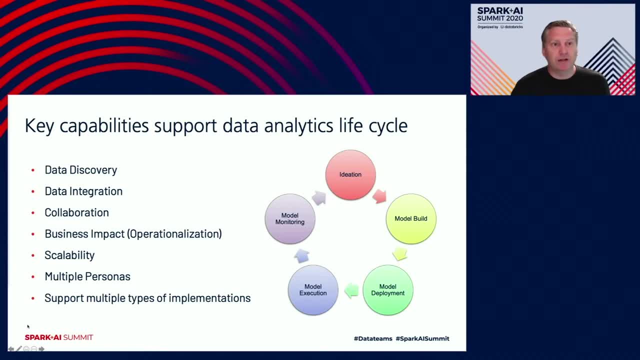 Other times it was fine for the business to know the next day or maybe once a week If it's something where it's a triage or a workflow type thing. we didn't necessarily need to know that instance and batch generally was easier and quicker to build and deploy. 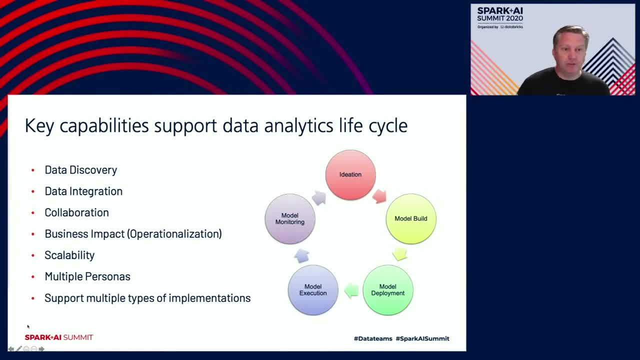 over real-time integrations And also scalability. Scalability can mean different things to different people. We need to make sure, from an analysis standpoint, we were using tools that allowed us to scale up or scale out the analysis, like the days of having data sets. that 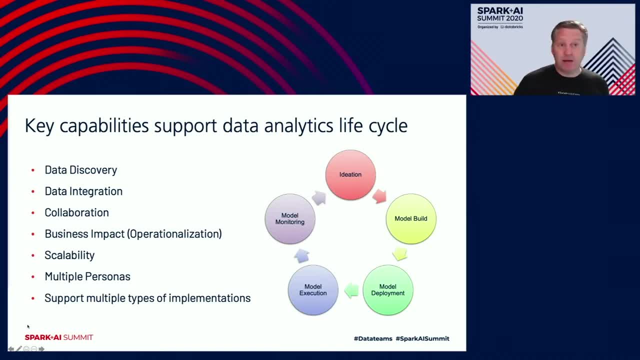 fit and work on your local desktop or laptop. Generally that isn't the case in enterprise settings, So we needed to make sure we could definitely easily scale up, scale out our compute needs And also, from a people perspective, we needed to make sure that we definitely preferred. 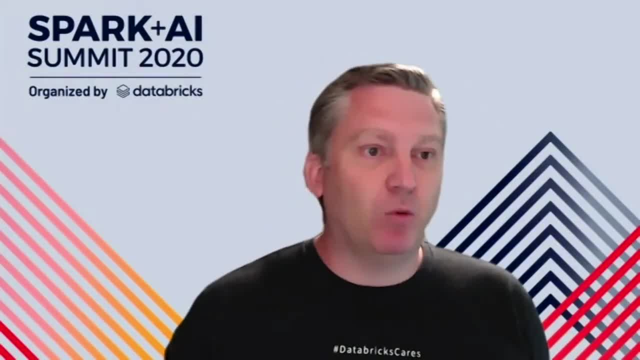 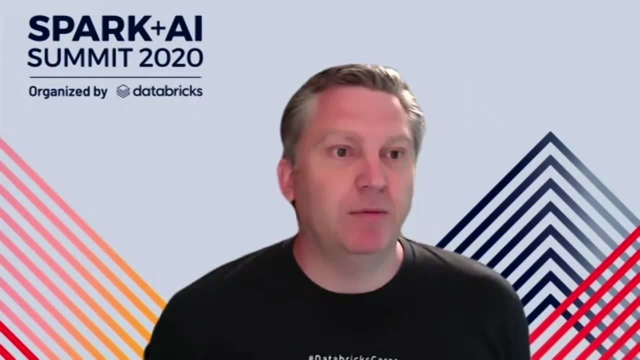 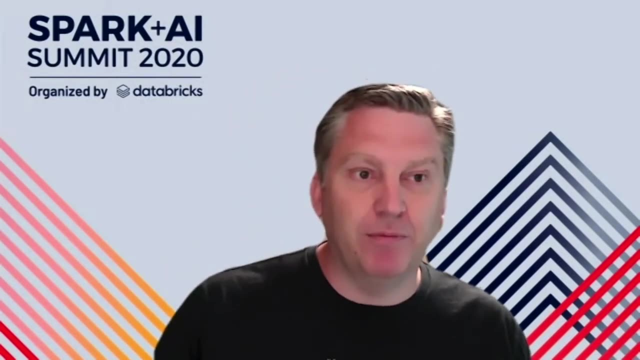 server-side web-based tools. So that way we didn't have to worry about enterprise setting. Your client environment might be locked down. So we needed to make sure We had tools that could scale out to a fairly large user base. And then deployments: we needed to make sure 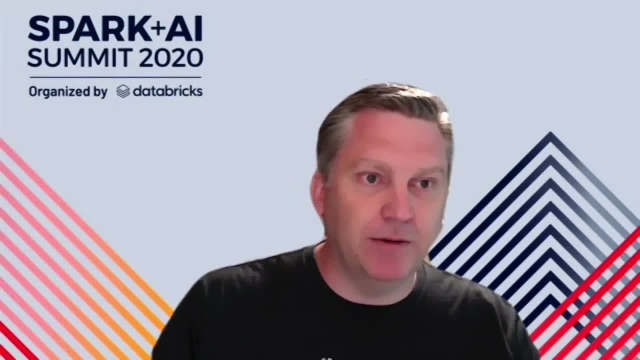 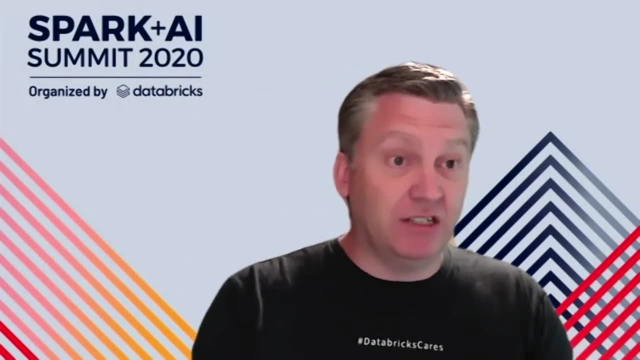 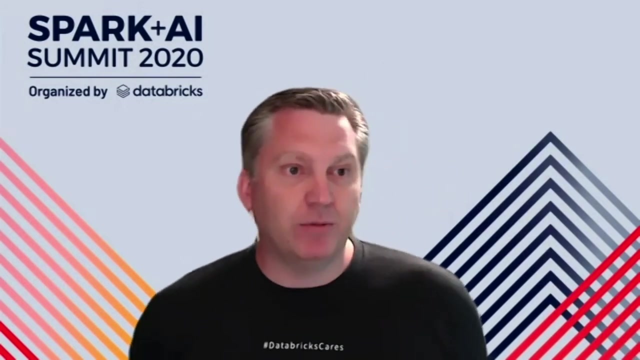 that we were using tools that we could actually take the work that was done by our data engineers or data scientists and be able to quickly move that to a deployment ecosystem. And now I'm going to kind of hand it over to you And Ming is going to kind of go into detail around some. 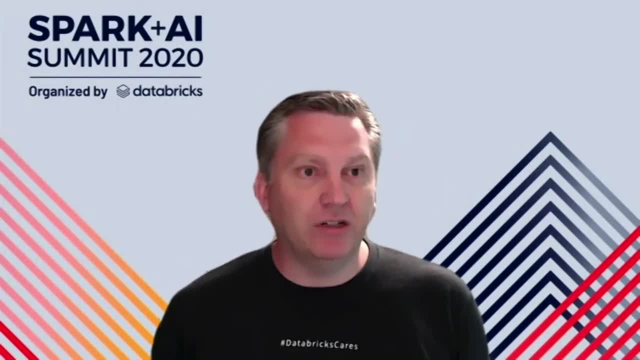 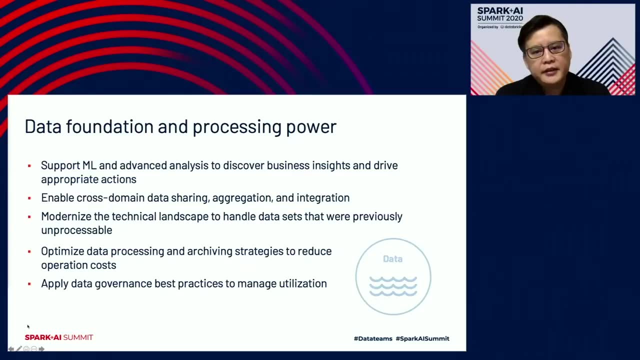 of our data discovery and integration capabilities. Thanks, Dave. So let's talk about the data foundation. To us, data foundation doesn't just mean the bytes on disk. Data scientists need a powerful platform where data can be stored, transformed and analyzed. 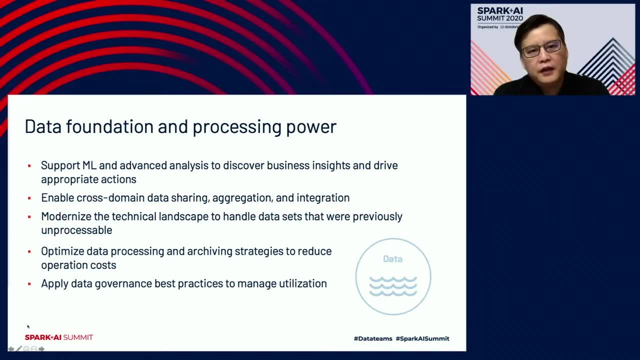 On the slide. here are a few use cases of the data platform. First of all, the platform should allow data scientists to apply mathematical algorithms to the data and generate insights. Those insights will, in turn, help Zurich and our customers to make better business decisions. 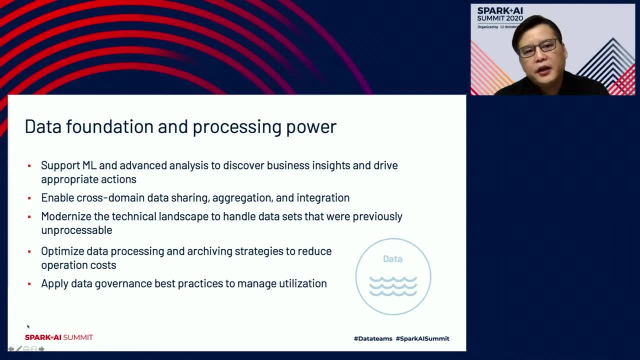 and drive business impact. After being curated, the data can serve for many purposes. The platform should also provide an avenue for business users to explore data, for data analysts to find hidden patterns and for the reporting analysts to create BI reports. The definition of analyzable data. 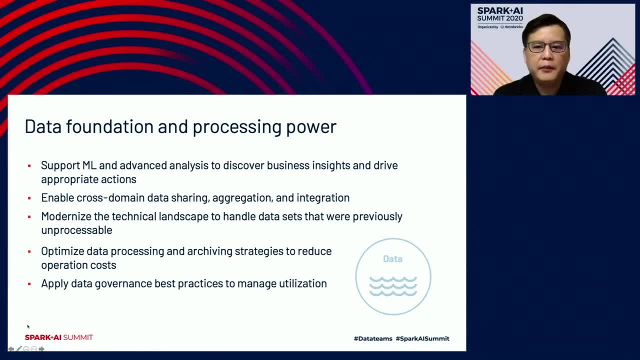 has changed from the corporate tabular format to all kinds: structured, semi-structured or even unstructured. The platform should allow users to map data. The platform should be able to match them up together and make sense of them. Other use cases include optimizing operational cost. 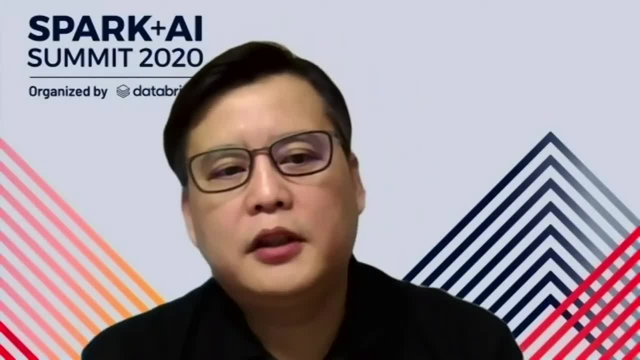 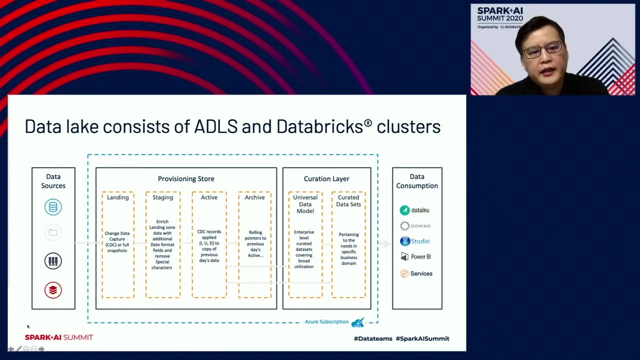 and support security and governance processes. In response to those use cases, Zurich has implemented a data lake on Azure Cloud. The lake concept has been around for a while. Using cloud services, our lake is not only the simple storage place, but also offers plenty of processing power. 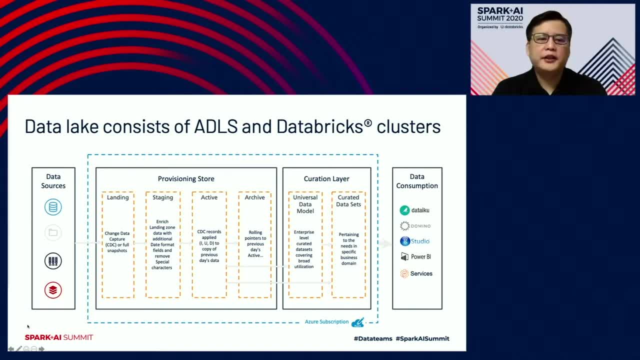 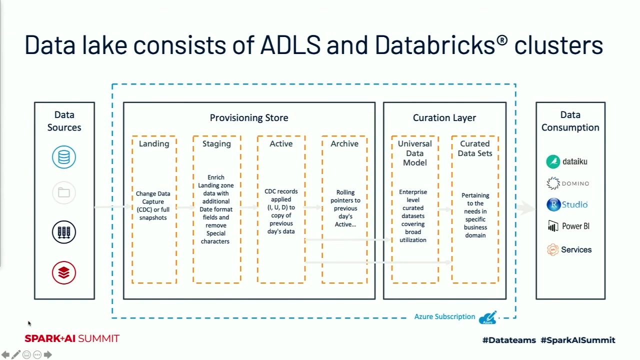 We divided the physical storage into separate layers. Just like water, data flows through those layers and gets purified for the consumer. The layered design aims to meet different needs from different groups. Each layer is a dedicated network location and the data files are further organized. 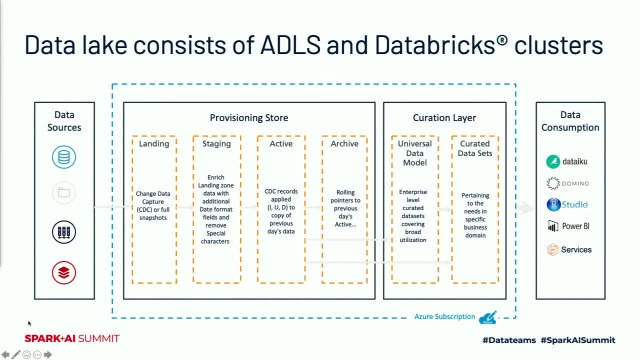 into folder structure by subject area source system and the timestamps. Spark cluster is the computation engine pushing data through those layers. The cloud provides multiple options to economically implement a data lake architecture. We store data files on Azure ADLS and use data breaks. 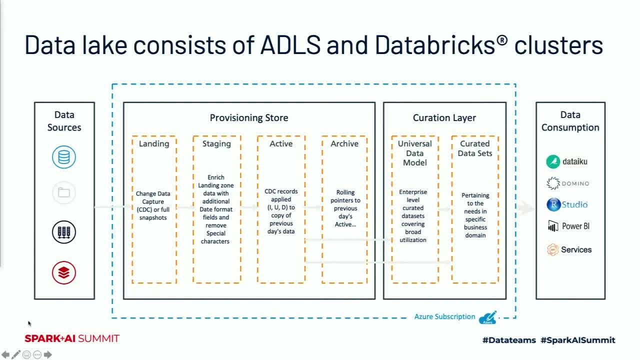 as a path offering. ETL pipelines are managed by an in-house developed framework. Currently, our data lake platform has more than 900 terabytes of data and performed more than 40,000 transformation tasks each day, And those numbers are still growing. 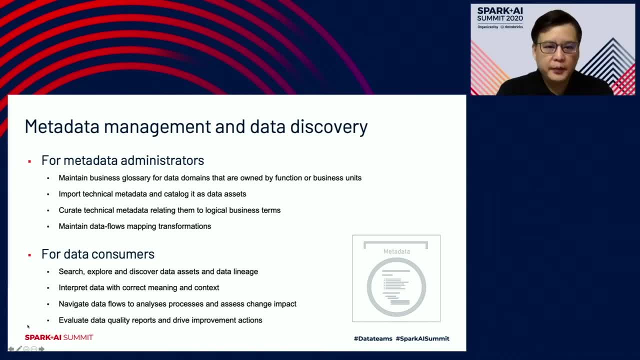 MatterData is a shorthand representation of a data. It makes finding and working with instance of data easier. Considering the size and complexity of our data lake, a platform supporting MatterData management became critical. We defined an admin role to collect and manage MatterData entries on the platform. 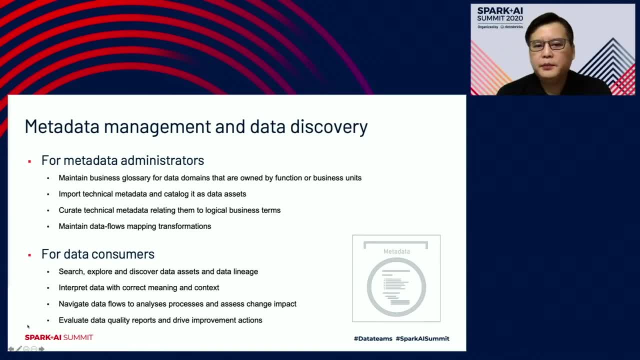 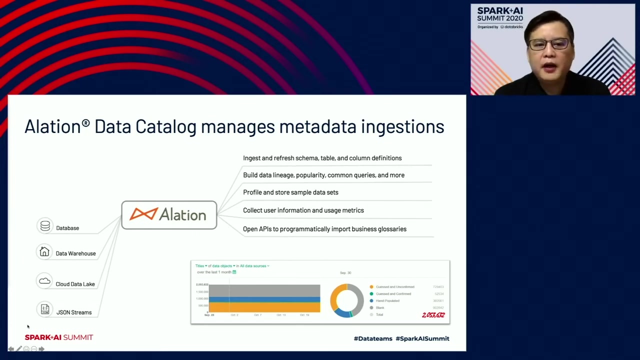 The other end of a platform is the user. They use the platform to search, view, use and share MatterData. We expect our MatterData management platform to facilitate all of those functions. After carefully evaluating several data catalog products, we chose Alition as the MatterData management platform. 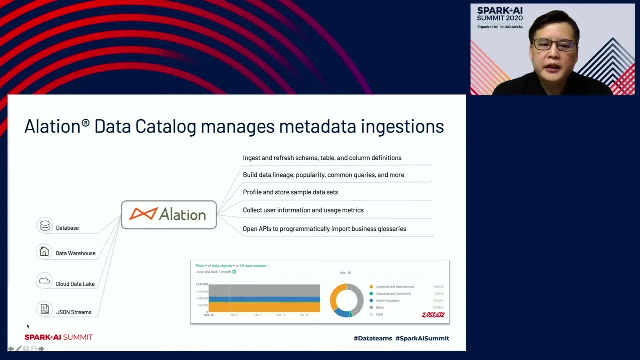 Using the built-in connectors. we quickly integrated Alition with the data lake plus 18 on-prem data repositories. The synchronization with source systems are automated and managed by Alition so that MatterData changes in those sources can be rapidly reflected. Currently, our Alition platform. 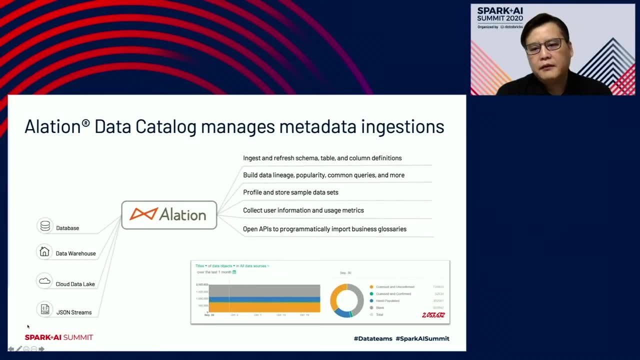 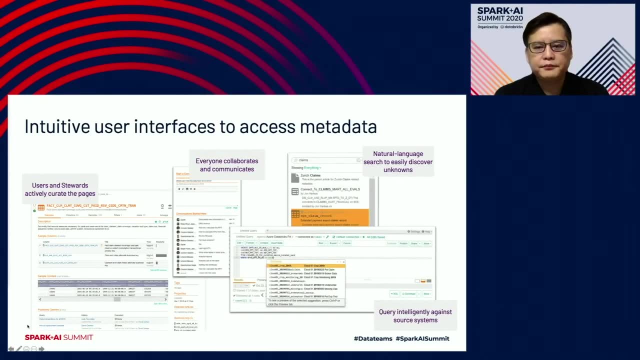 has more than 2 million MatterData records covering 1.4 million data, And we have over 4.5 petabytes of data. Alition's UI is easy to use. MatterData info is well organized in web pages. We have enabled the social collaboration features. 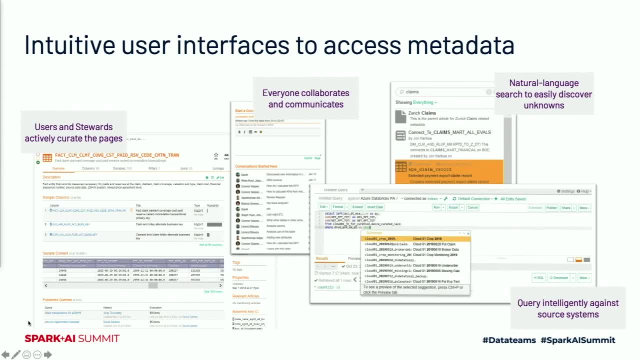 such as Google search endorsement, object watching and alerting. A built-in SQL editor would allow to quickly pass ad hoc SQL queries against any source system. All these are front-end functions. makes the data catalog a self-service portal of the entire data ecosystem. 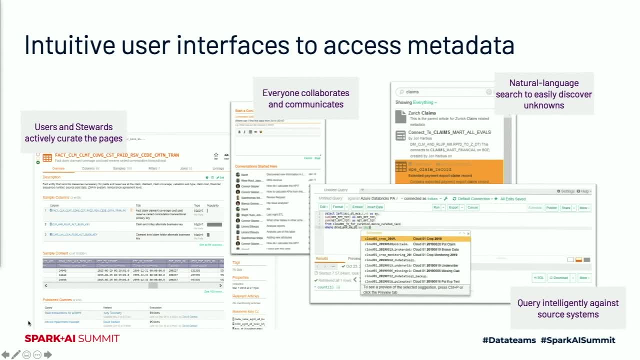 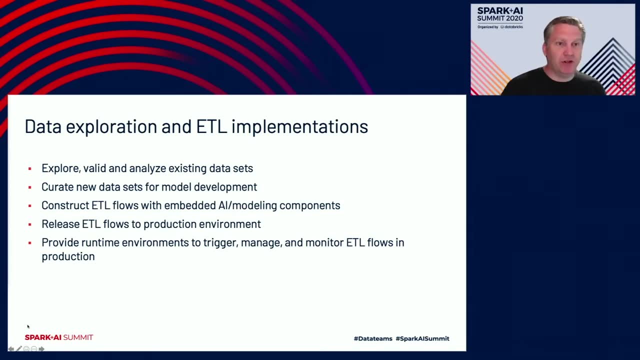 Now I'm turning to Dave to talk about the next platform. Thanks, Ming. So, as Ming talked about our data discovery, we wanted to make sure, as we were looking through our data log and our data scientists analysts found additional information about a given data source, be able to contribute that back. 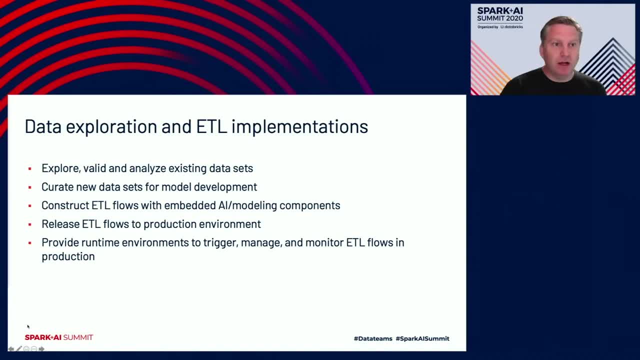 but also then be able to pull that into an overall ETL pipeline and training as well. as for scoring And the way that we did that, we leveraged multiple tools which kind of have a flow. we'll kind of go over in a bit. 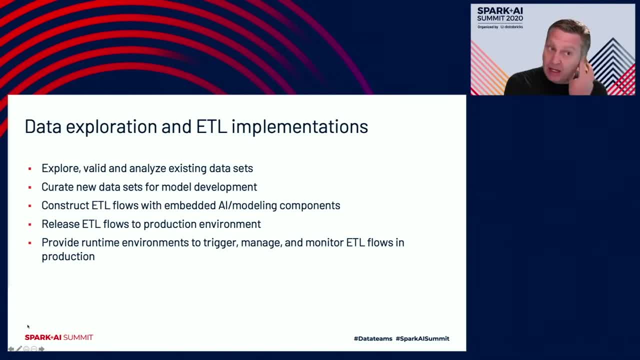 but we wanted to make sure that we eliminated a lot of the silos that we had historically, where our data analysts might want to use a SQL-based tool, or people who really wanted to use R would use like RStudio, or we would have people that maybe had a smaller data set. 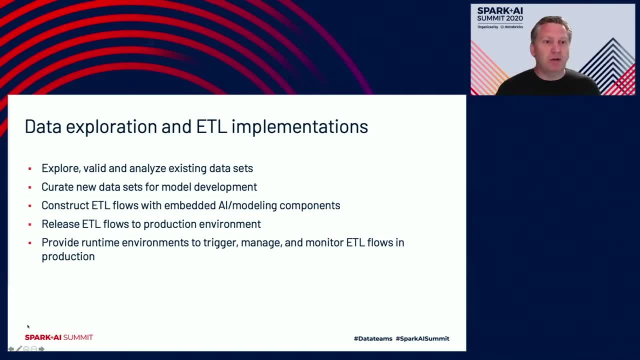 and they want to use Python. they might just be using local Jupyter. Well, what would happen is, on larger projects, we would have different portions being worked out and analyzed separately. They might copy over the resulting data sets and integrate them together. 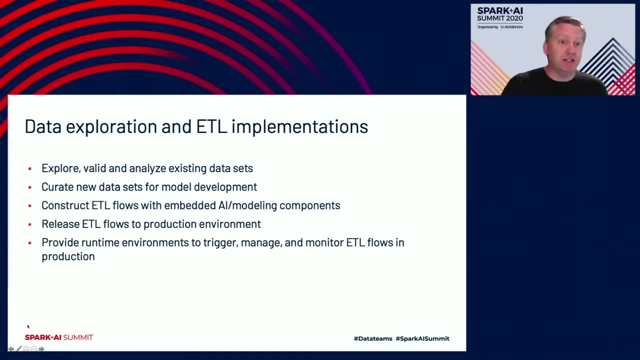 but we kind of lost potentially on some projects that full, in the end at least, from an ease of integration. So to the extent, if we had to like stitch this into a common pipeline, we had to once again refactor all of that into a common pipeline. 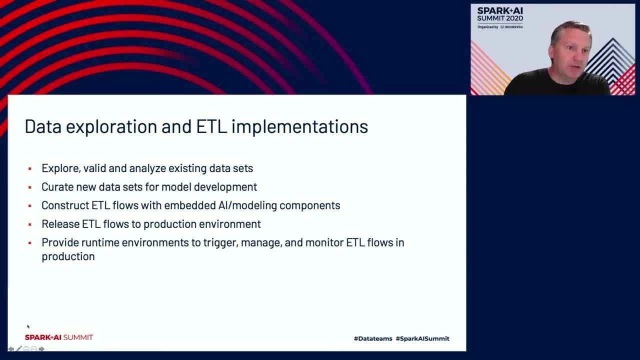 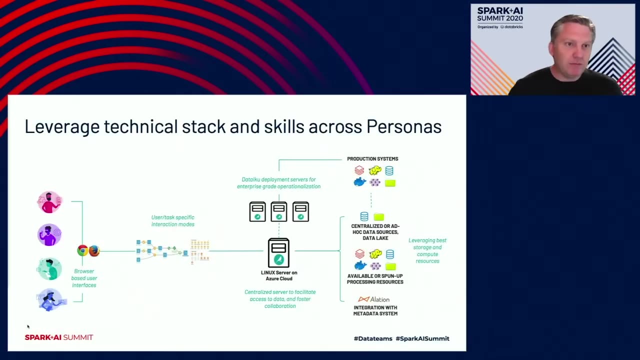 which really slowed down and had tremendous impact on our speed to market. So we wanted to make sure that we really could help those multiple personas that we talked about before really work together and integrate into an overall pipeline. So this is just like a really high level view and flow. 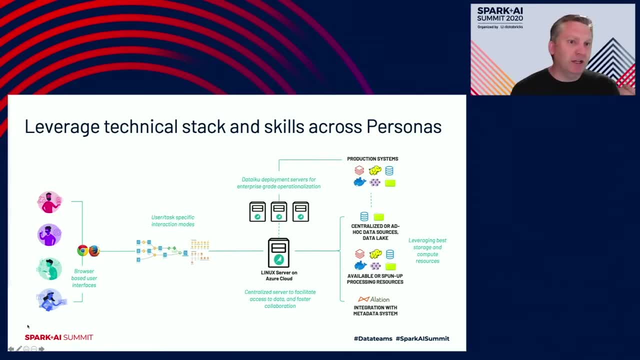 of that. hopefully, one thing you got out of this is like the integration, Like we needed to easily facilitate the integration of various data sources. Like I've been saying, we had a cloud data lake, but we still had a lot of on-prem historic data sources. 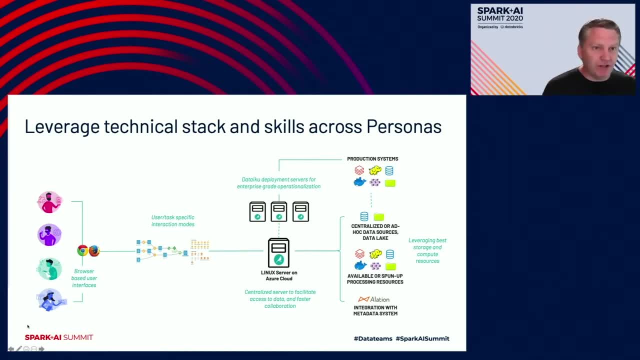 that. maybe they're in a teaser, maybe they're Microsoft SQL Postgres- what have you? And we didn't want to have our data scientists be wasting cycles on tracking down not only the right drivers but also the right credentials. I'm sure this only happened at Zurich. 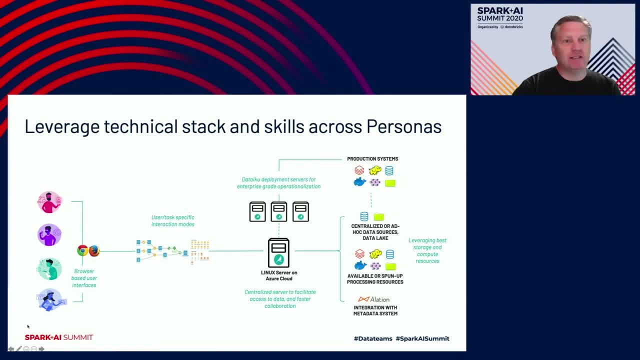 Everyone's done it- where they accidentally maybe put secrets into like a code repository or something like that. We wanted to make sure that the right way was the easy way right, So we leveraged as our front end integration tool Dataiku and that kind of allowed people who wanted to work. 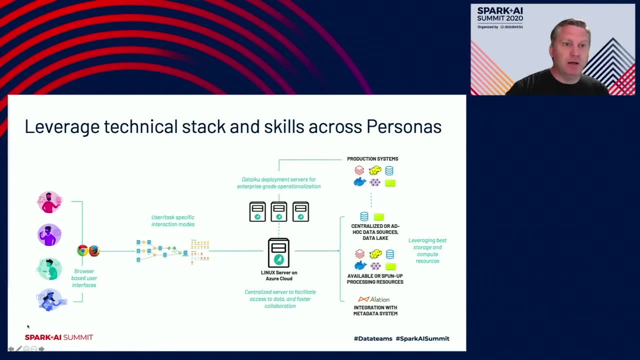 with like a code list, code light, type, environment or maybe even SQL or R, push a scale of competition out to a spark layer, allowed us to build that out in a way that we capture all those business roles. But we also were able to then take that and bundle it. 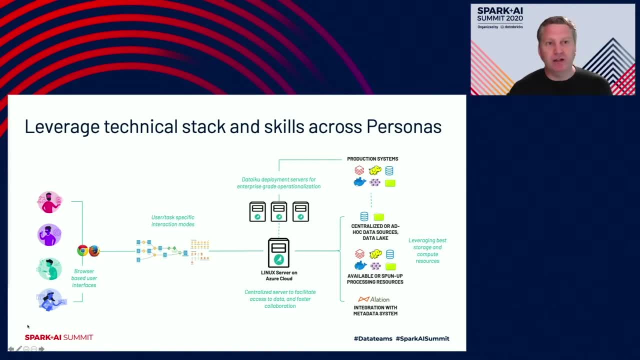 and test and push it out to production And our timelines went down from tens of months to a matter of months, which, compared to what we were used to, was huge to our business and also helped us support, like the multiple types of deployment where 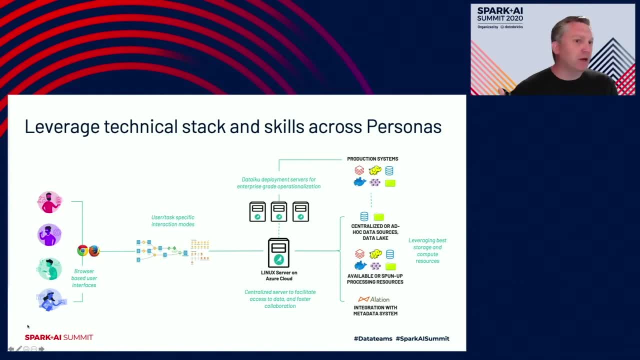 to do the initial business impact. you might do a more simple deployment, batch deployment, and then work on maybe the more robust or the real time type deployment solution And as far as like other options of deployment, Ming is now gonna be covering that through our use. 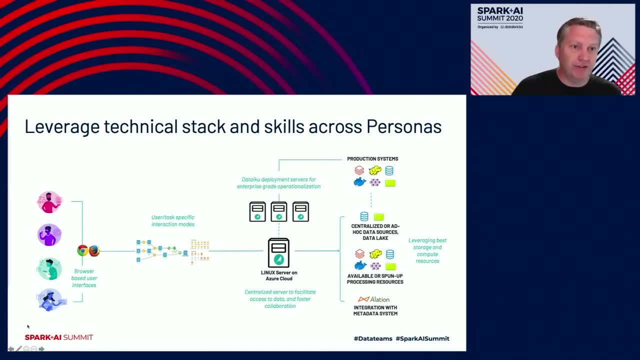 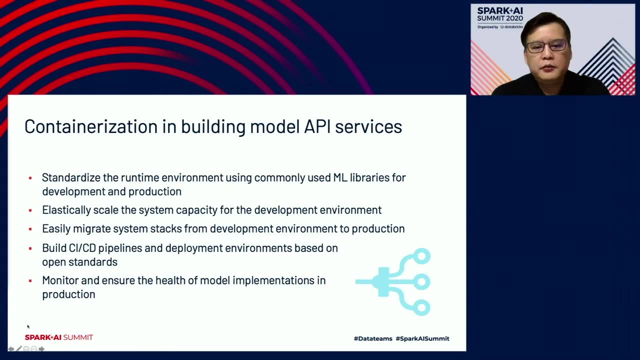 of containerization and CI CD processes. Thanks, Dave. Let's switch gears to model deployment with containers. Containerization is a lightweight virtualization mechanism. A container can be easily created from a manifest file And the precisely encapsulate the application with its own runtime environment. 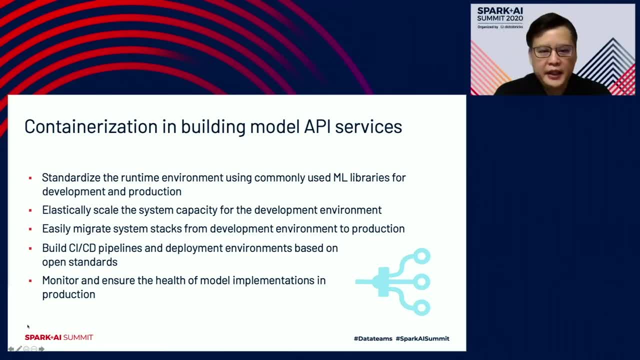 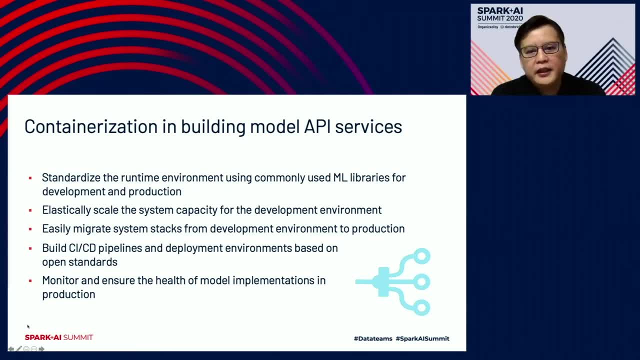 The container platform also naturally support elasticity. The instances can be rapidly provisioned or deprovisioned to adapt to the workload changes. This is really useful to economically maintain the right system capacity. Containers are immutable packages and can run virtually anywhere, So we can easily migrate a containerized application. 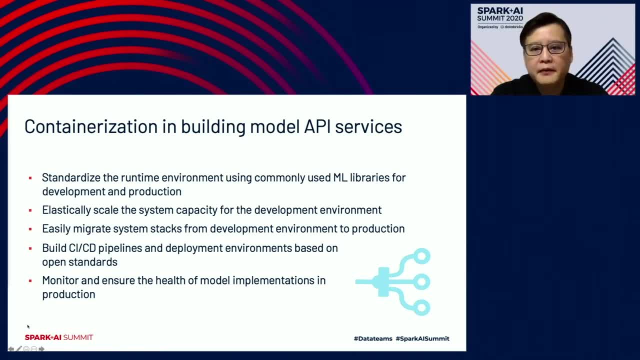 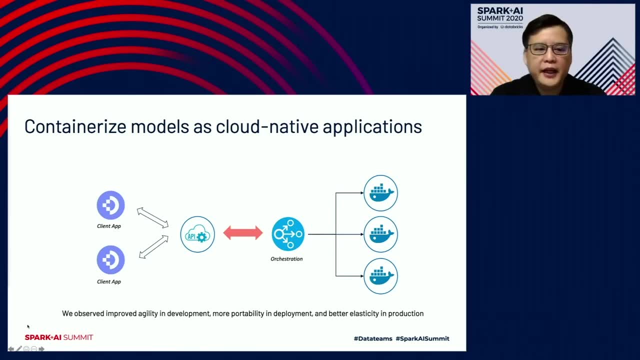 from development to QA to prod Along with the container. we often heard microservices. This term referred to an architectural style, A set of small services communicate with lightweight mechanisms. Each service run in its own process and can be independently or independently. 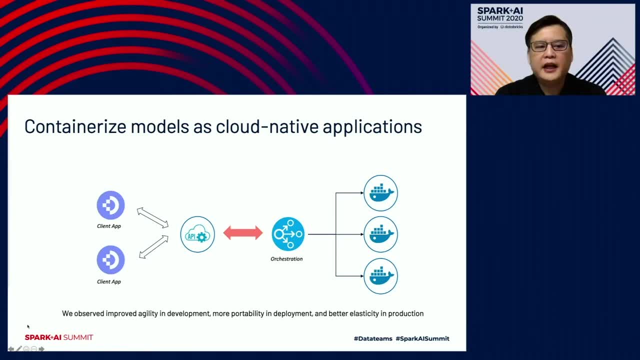 distributed And the. We see microservices as a good fit to implement scoring engine APIs, As Dave mentioned before. The diagram on the slide is our reference architecture where we tied microservices containers and the cloud together. The diagram on the slide is our reference architecture where we tied microservices containers and the cloud together. 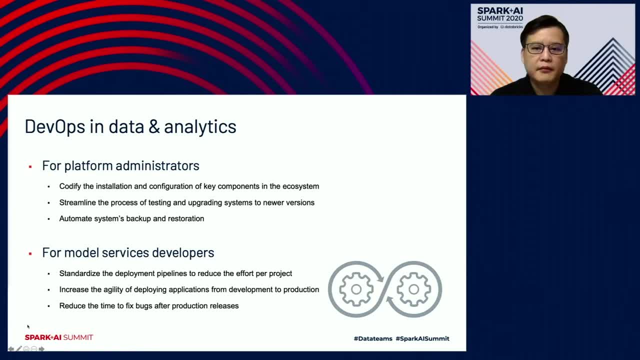 The diagram on the slide is our reference architecture where we tied microservices, containers and the cloud together. DevOps is a methodology where development team and the opt teams work closely, from design to development to production support. This collaborative approach promotes the productivity. 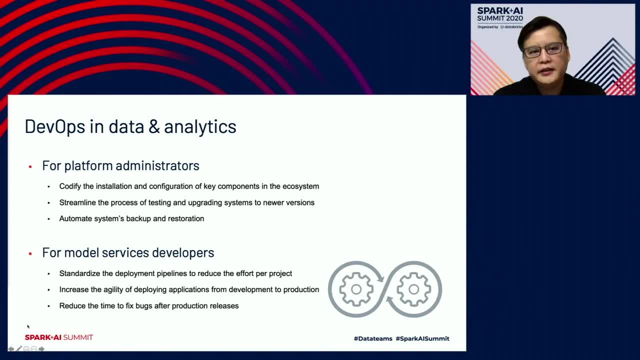 so that IT teams build tasks and then release software faster and more reliable. This collaborative approach promotes the productivity, so that IT teams build tasks and then release software faster and more reliable. While working on our data platforms, we have successfully introduced the DevOps principles to the field of data and analytics. 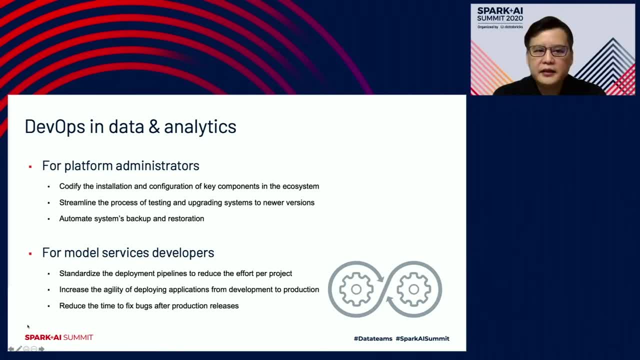 The data scientists and IT teams start collaborating as soon as a new project kick off. Push button deployment enable us to iteratively release new versions, and even business users can also participate in the process. They could test and give feedback right after each release.